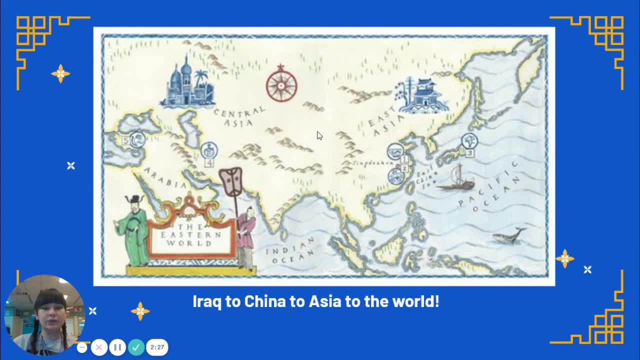 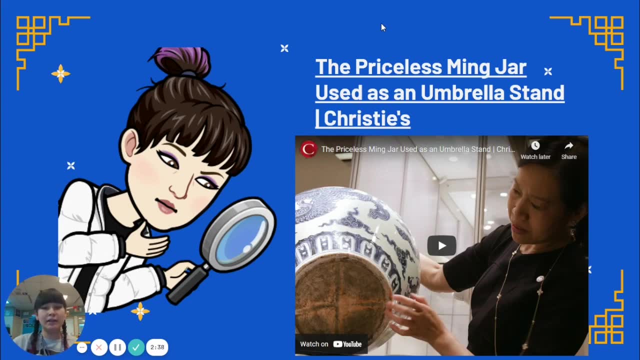 We are always inspired by other artists and other cultures. Because the Ming vase style is so popular around the world, a lot of them are fake or made recently, So they are not actually from Ming dynasty, But sometimes people have rare finds of these Ming dynasty pottery. Here's an example of 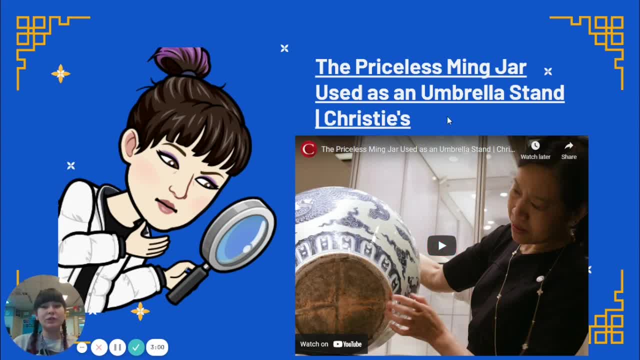 a Ming vase that somebody bought at a garage sale and used as the umbrella stand. And then they'd be, And then they realized that it was actually a real Ming vase used by a king in the Ming dynasty, And this vase turned out to be worth $20 million. 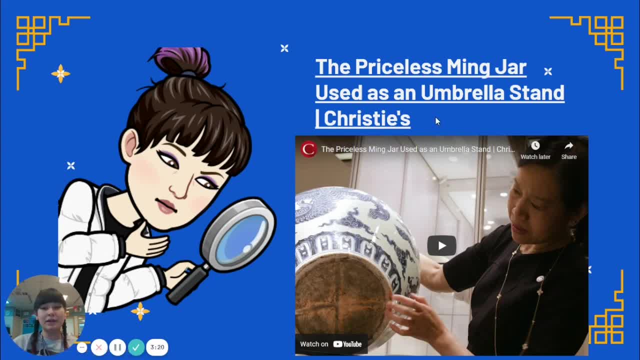 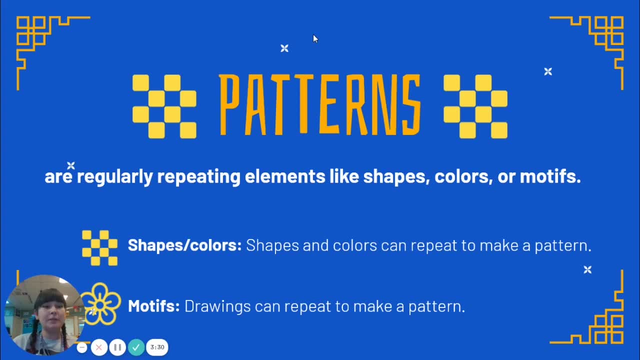 I will leave a link of this story in this week's assignment. If you're interested. you can watch that as well. With this project, we're going to be looking at the principle of design patterns. Patterns are regularly repeating elements such as shapes, colors and motifs. 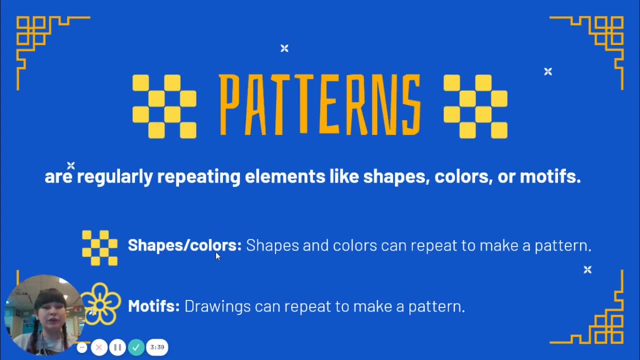 We always talk about repeating shapes and colors when we do patterns, And when shapes repeat or colors repeat, it can become a pattern. If you have stripes- red, red and blue, then it would be red, blue, red, blue repeating. 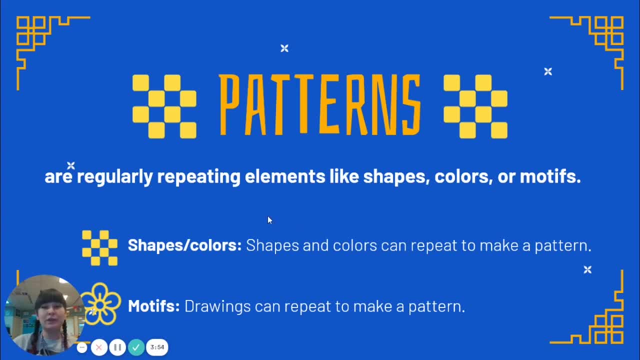 If you had a pattern with squares and circles, it might repeat: square, circle, square circle, And that is a pattern that we have talked about. Patterns can also be made with motifs. Motifs are little drawings that repeat over and over. 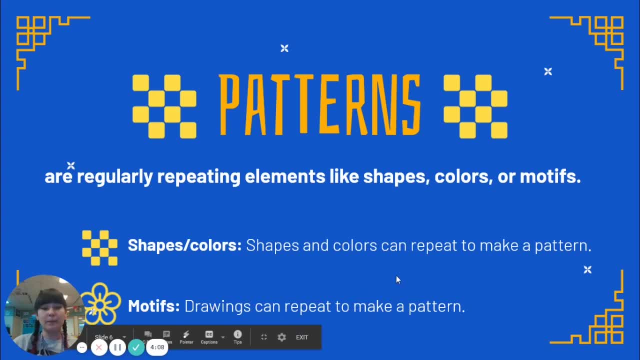 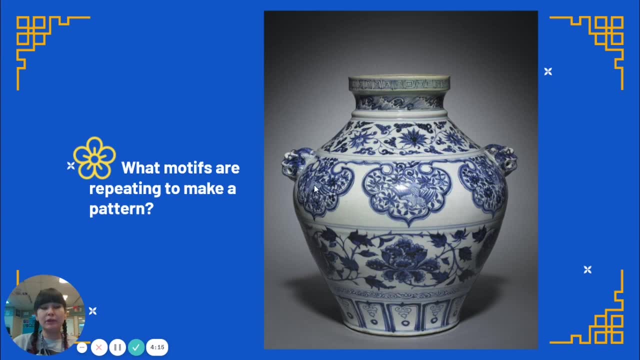 So drawings can repeat to make up patterns. If you look at this Ming dynasty vase, you see that the motif of birds are repeating. There's one here, repeats here and repeats here. There are different border designs that repeat The designs up here are repeating over and over. 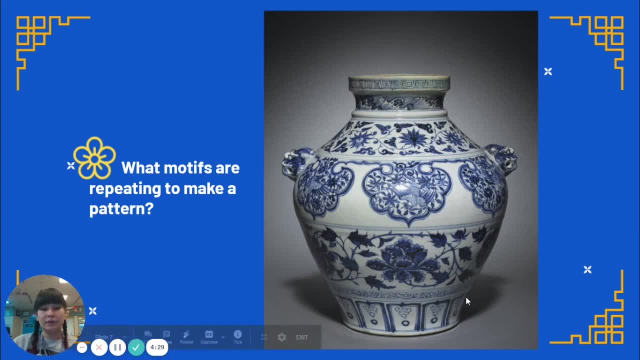 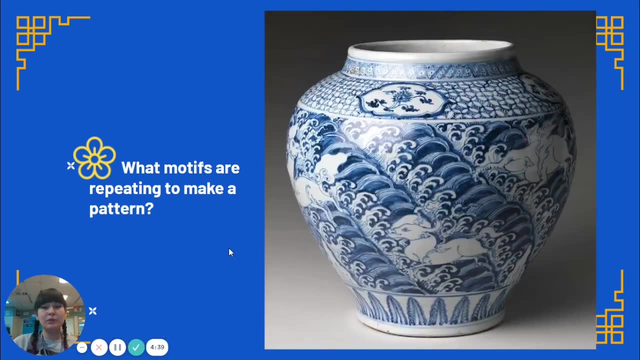 The waves are repeating. What else do you see that's repeating? You might see vines, flowers repeating more designs. What motifs are repeating? We see that the flowers are repeating in this one. The waves are repeating. The animals are repeating. 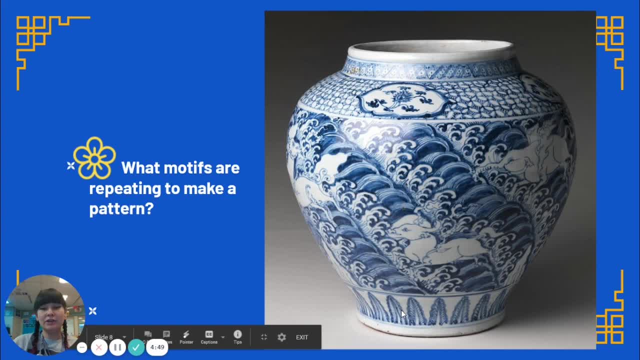 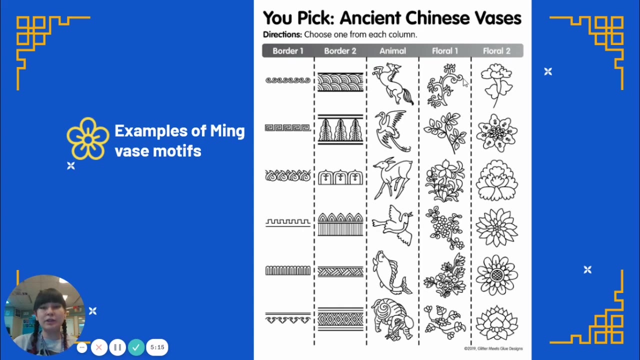 The flowers and the designs on the bottom are also all repeating And they're all very detailed. Patterns and details are very important part of Ming vases. In this week's assignment I also have a handout that has different types of borders animals.